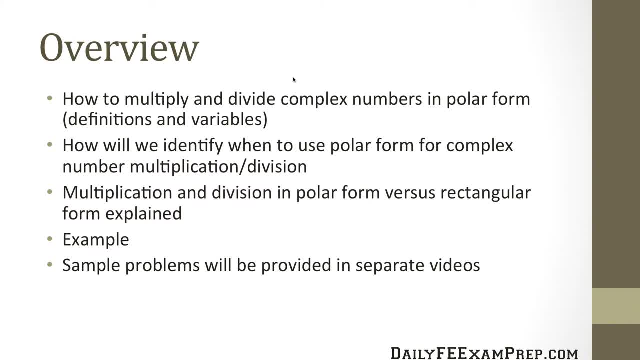 Any additional sample problems. we do have some that will be provided in separate videos. So if you need some extra help, be sure to check out for that. And just as an added bonus as well, multiplication and division of rectangular form of complex numbers are available in the downloadable lesson plan for the members content. 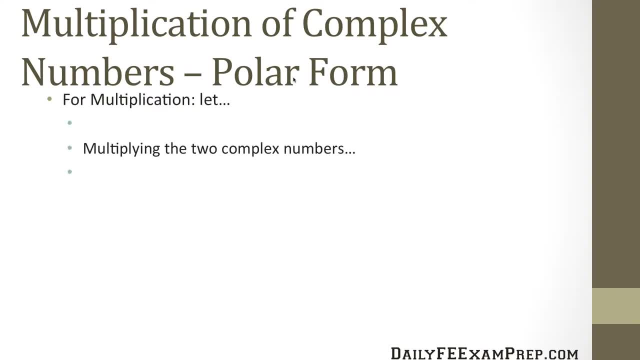 Okay, so multiplication of complex numbers in polar form. So for multiplication, let z1 equal r1 angle theta One and z2 equal r2 angle theta two. now, multiplying the two complex numbers, we get z1 times z2 is equal to r1 times r2 angle theta one plus theta two. 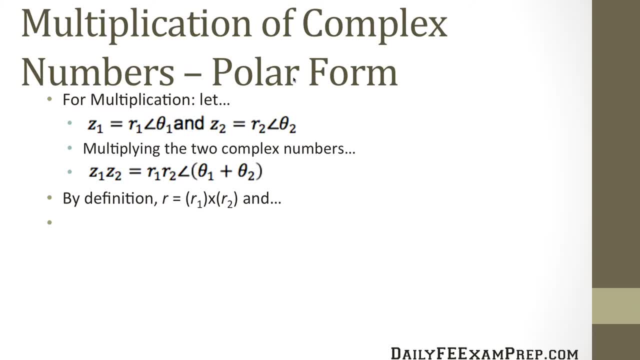 Now, by definition, r is equal to r1 times r2 and theta is equal to theta one plus theta two. so that's kind of where we get that derivation from. that gives us the r1- r2. an angle Michaela �데 pond of angle theta. OK, let me show you what that is. 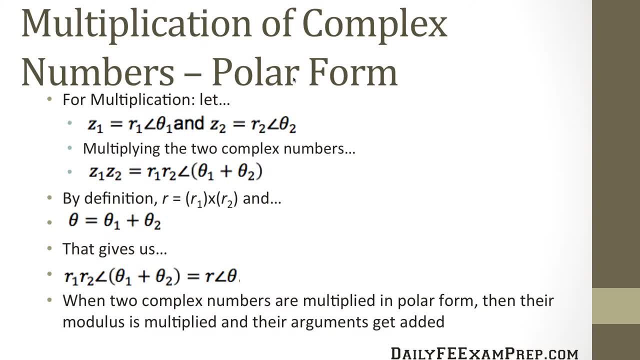 Beta 1 plus theta 2 equals r1 times, or, excuse me, r1 point and angle theta. so when two complex numbers are multiplied in polar form, than their modulus is multiplied and their arguments get added. So be sure to recognize the difference then, because they're not both multiplied. 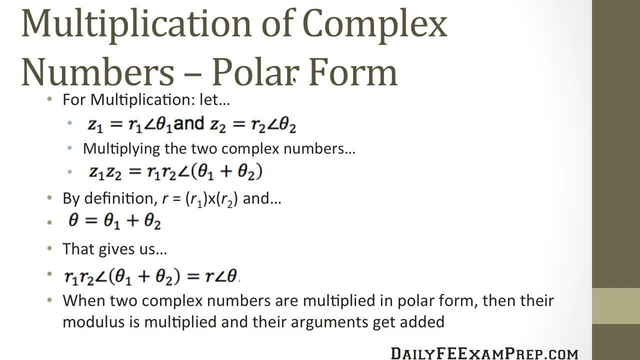 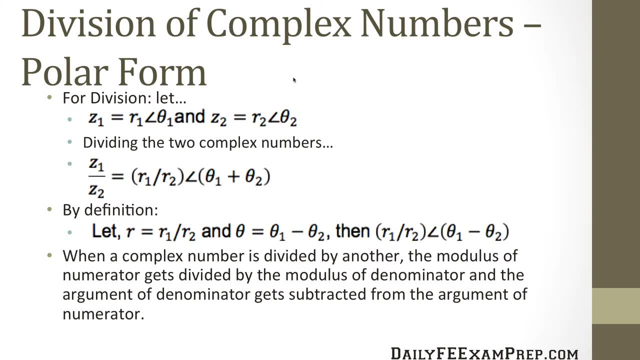 And so you have one that's multiplied and then another set that's added. So be sure to be sure to note that down. OK, complex numbers in polar form. we let Z1 equal R1 angle theta 1 and Z2 equal R2 angle theta 2.. 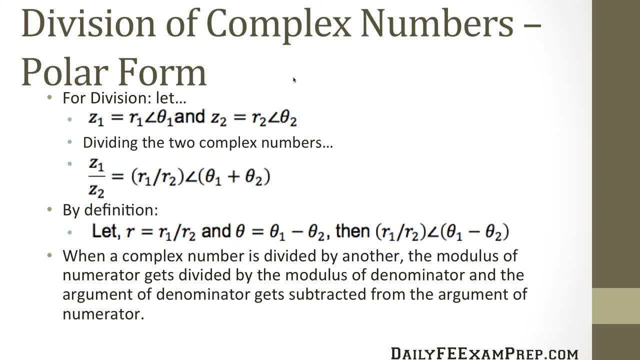 Now, dividing the two complex numbers, we get Z1 divided by Z2.. That equals R1 divided by R2 and angle theta 1 minus angle theta 2.. So make note here, this is just a typo That's supposed to be minus. So theta 1 minus theta 2.. So a little bit further explanation by definition. 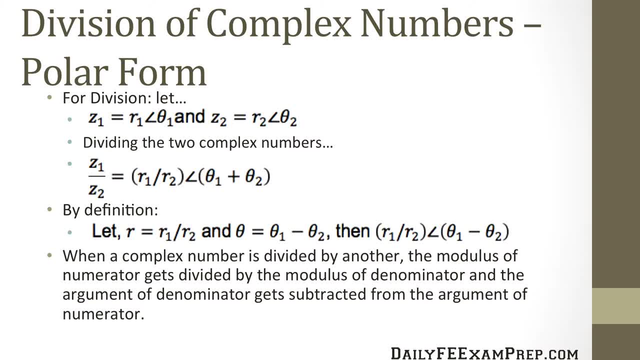 if we are dividing, then we get: R is equal to R1 divided by R2 and theta is equal to theta 1 minus theta 2.. So that's what gives us that Z1 over Z2 definition. So when a complex number is, 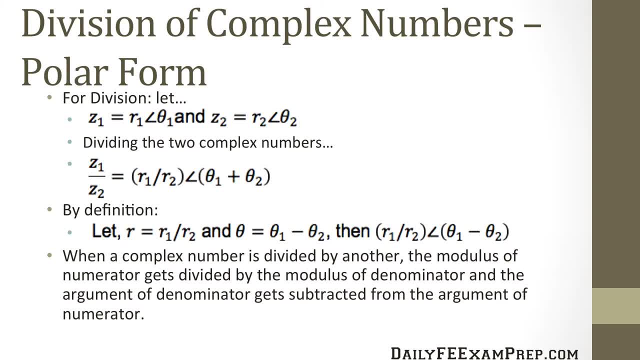 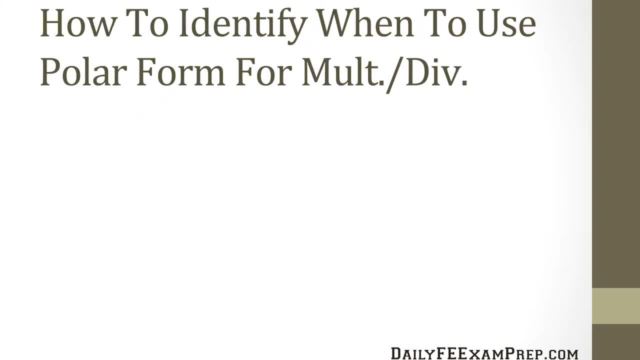 divided by another. the modulus of the numerator gets divided by the modulus of the denominator and the argument of the denominator gets subtracted from the argument of the numerator. Now how do we identify when to use polar form for multiplication and division? Well, multiplication and division can be carried out. 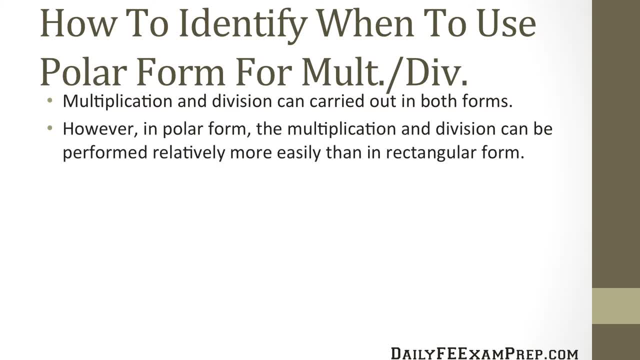 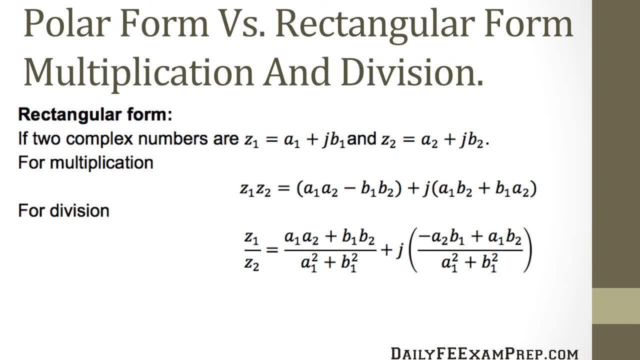 carried out by the denominator and the argument of the denominator In both rectangular and polar form. However, in polar form the multiplication and division can be performed relatively more easily than in rectangular form. So polar form versus rectangular form. multiplication and division is described like this. So the rectangular form. if two complex 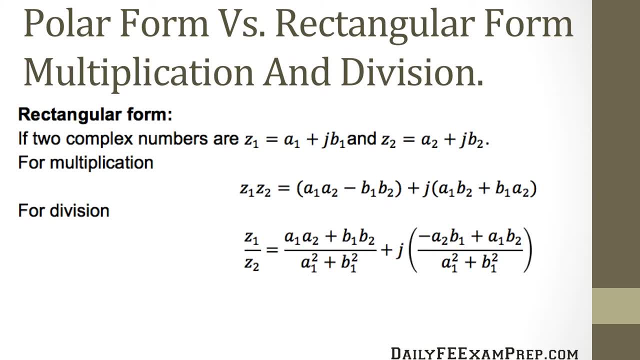 numbers are: Z1 equals A1 plus J times B1, and Z2 is equal to the A2 plus JB2, then, as we discussed before, Z1 times Z2 is equal to A1 times A2 minus B1 times B2 plus J times A1B2. 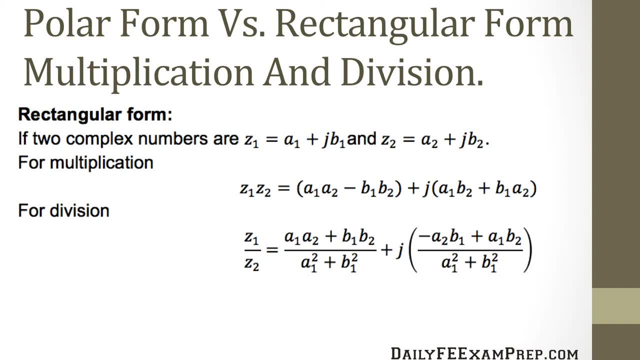 plus B1A2.. Now for division. we have: Z1 divided by Z2 is equal to A1A2 plus B1B2 divided by A1 squared plus B1 squared plus B1 squared. So we have: Z1 divided by Z2 is equal to A1A2 plus B1B2 divided by. 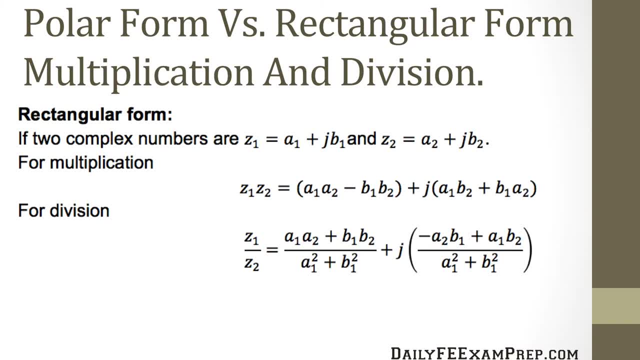 A1A2 plus B1A2 plus J times minus A2 times B1 plus A1 times B2, divided by A1 squared plus B1 squared. Now that was pretty complicated in the rectangular form, which is why we try to push. 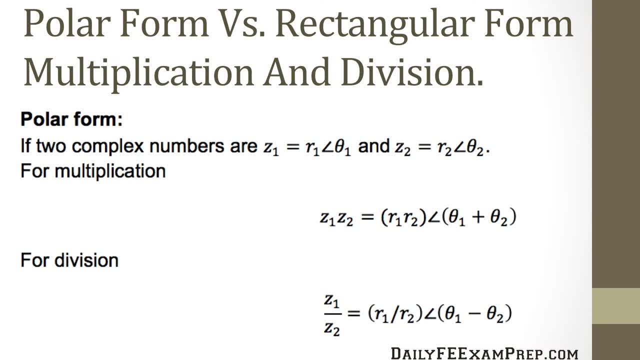 everybody towards the polar form for multiplication and division. Now, in polar form, if two complex numbers are given as Z1 and Z2, we have: Z1 equals R1, angle theta one, and Z2 is given as R1 angle theta two. So we have: Z1 equals R1, angle theta one, and Z2 is given as R1 angle theta two. 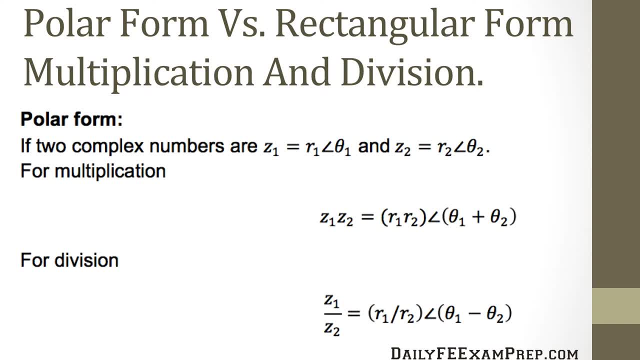 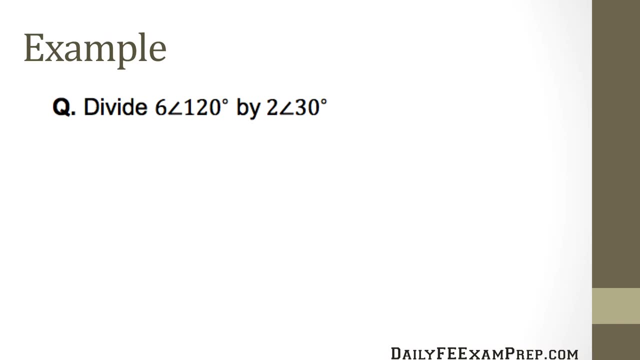 So for multiplying, like we just discussed, we have R1, R2, angle theta one plus angle theta two And division is just R1 over R2 and point theta one minus point theta two. So let's go through a quick example: Divide six angle 120 degrees by two at angle 30 degrees. So the solution that we 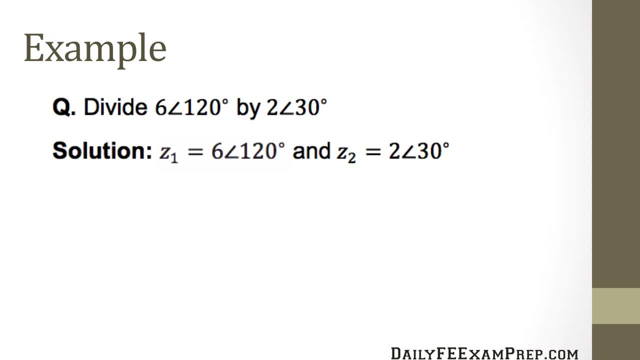 have here we have we define our Z1 and our Z2 values. Z1 is equal to R1 angle theta two. So we have: Z1 is six angle 120 and Z2 is two angle 30. So we use the formula for polar division given on.